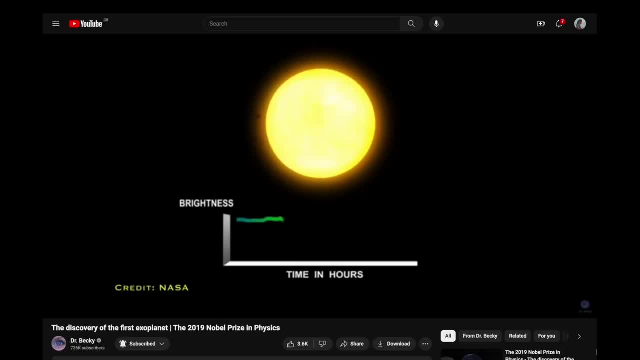 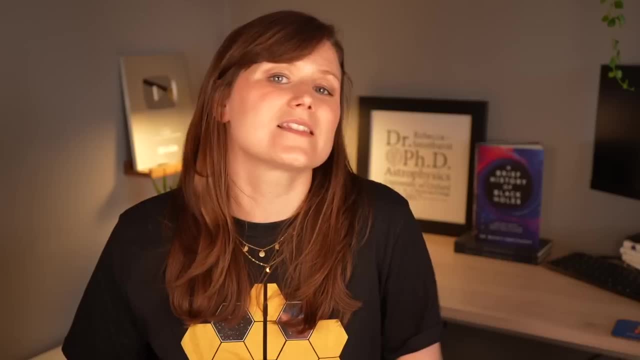 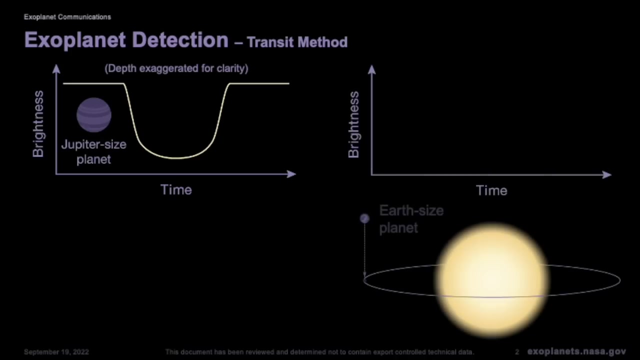 the wobble method. I put all of these in my History of Exoplanets video. if you wanna know more, I'll link that video in the description below. But TESS and its predecessor, Kepler used what's known as the transit method: monitoring stars for regular dips in their brightness because a planet has passed. 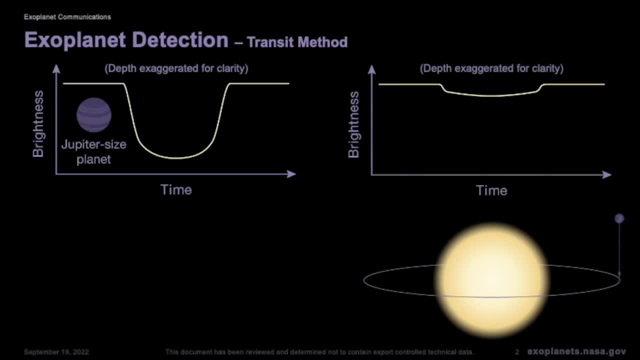 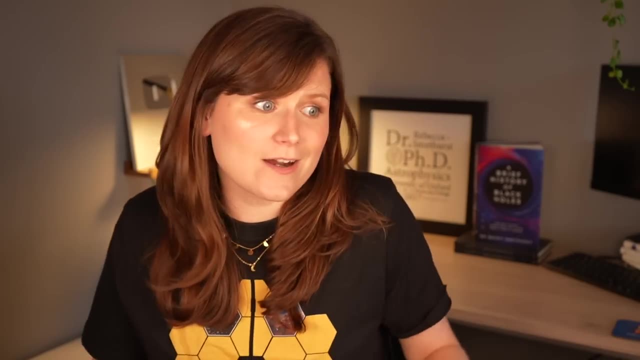 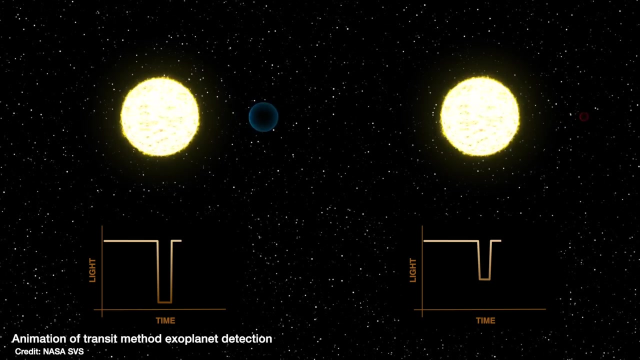 in front of that star on its orbit. from our perspective here on Earth. Again, this is a lot easier when you've got a big planet or one that orbits very close into its star, or both, because the way that planet is going to block more light, causing a bigger dip in the star's brightness. 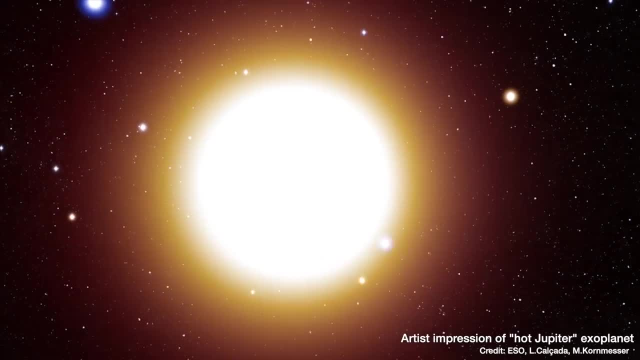 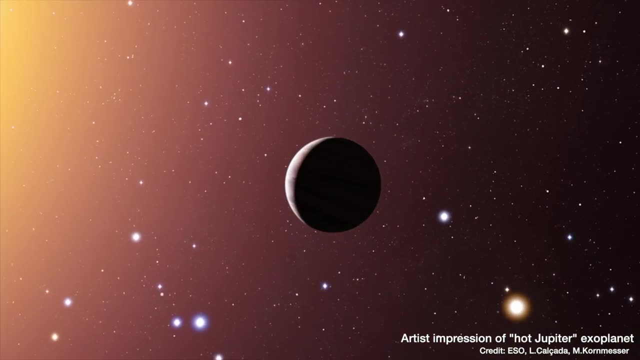 This is why so many exoplanets we know of are hot Jupiters, Jupiter-sized, but orbiting very close to their star, where it's much hotter, because they're just easier to spot. Plus, if the planet orbits close into its star, then its orbit's going to be really short. It might only take a few days. 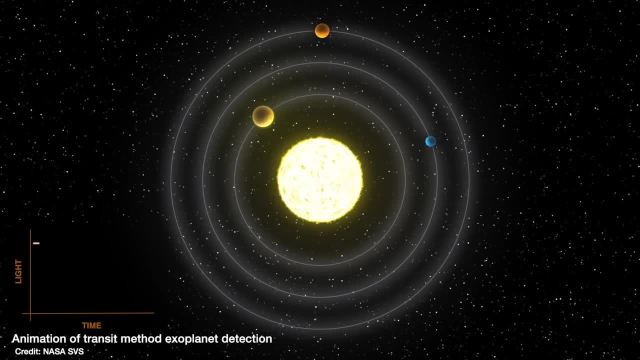 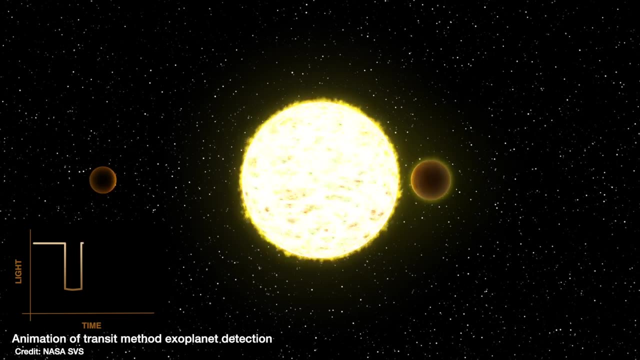 weeks or months to make one loop of the star, which means that you're only going to have to wait a few weeks or months to see that planet pass in front of its star again and confirm that dip in brightness that you saw was actually due to a planet and not some variation in the star itself like a star spot. That's why it's so hard to spot earth-like planets around sun-like stars that are in the habitable zone, because for them to be there you have to have a similar orbit to earth, and so you have to wait around for a year to see that very, very faint dip in the star's brightness again to confirm that the 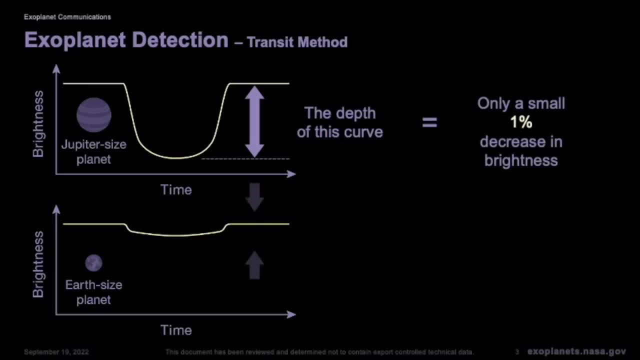 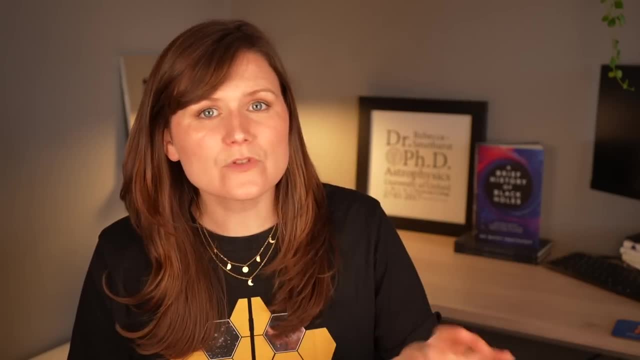 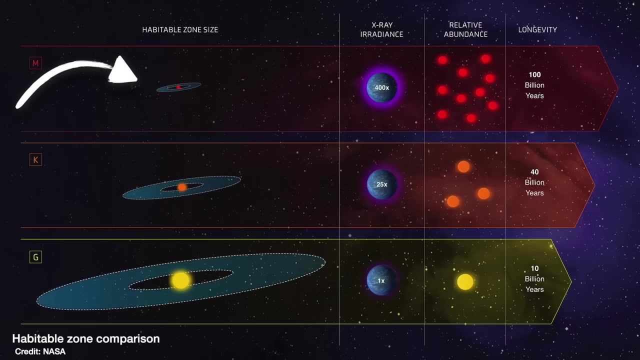 planet is there And we're talking about a tiny fraction of a percentage of the star's light for that dip in brightness. So that's why the majority of habitable zone rocky exoplanets that we know of have been found in orbit around M dwarf stars, Stars much cooler and smaller than the sun- around about 10%. of the sun's mass Being smaller stars. it means that the planets block an overall larger fraction of the star's light Plus to be in the habitable zone because the star's much cooler. it means they have to orbit much closer in, and so their orbits only take, yeah, a few weeks or months, which means you don't have to wait around. 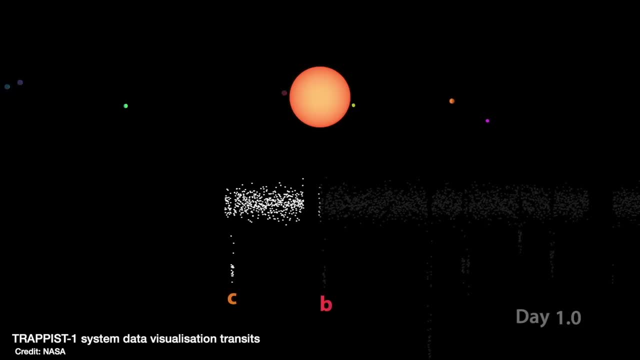 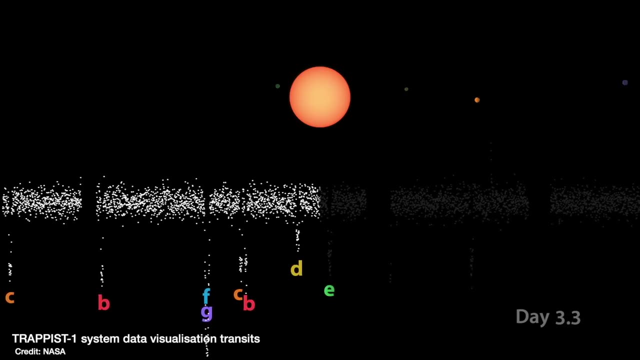 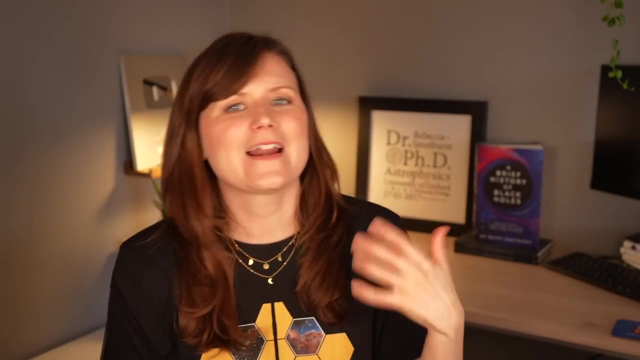 very long to spot the regular pattern in the dips of the star's light that they cause. For example, the famous Trappist-1 system of seven rocky planets are in orbit around an M dwarf star. There's a lot of unanswered questions, though, when it comes to whether planets in orbit around M dwarf 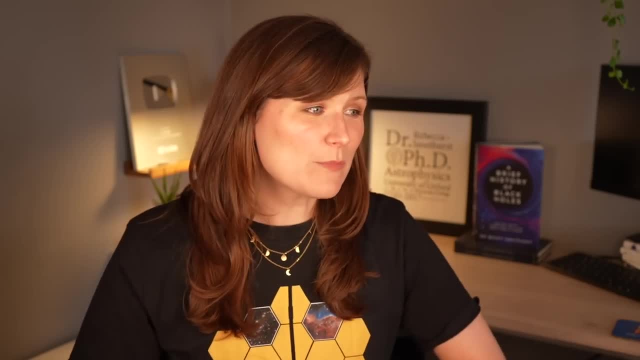 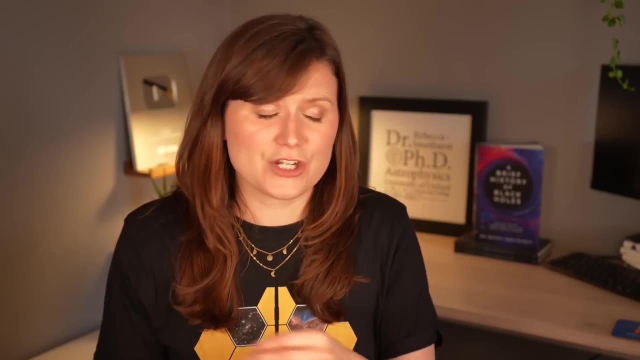 stars would actually be habitable Like there's some people that argue that M dwarfs are just too active and that they can flare huge amounts of high energy radiation that would just irradiate a planet, Maybe even completely strip it of any atmosphere and make it completely inhospitable to life, But then there are other people that argue that those flares could actually be the catalyst for biological processes that are needed to kickstart life. We're not going to know which of scenarios is the right one, though, unless we find more planets in orbit around M dwarf stars and try. 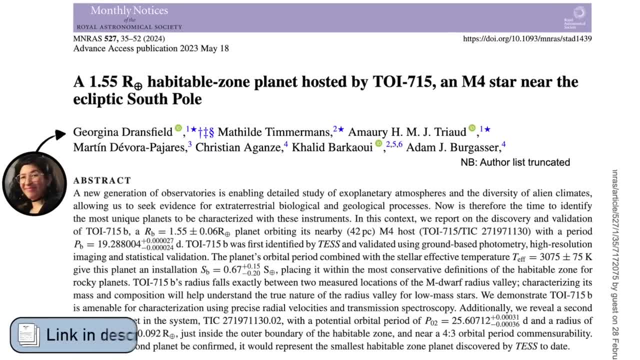 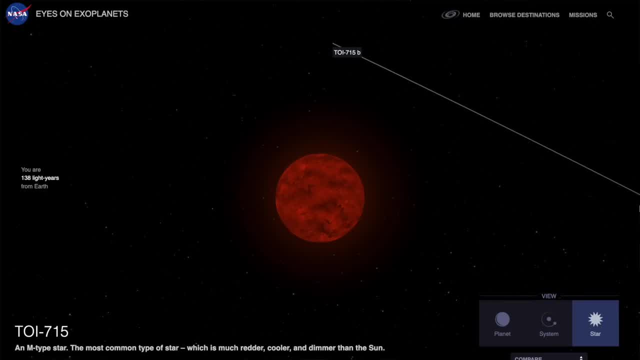 and study if they are habitable. So it's a good job that Dransfield and collaborators have done just that this past month using TESS. So they were monitoring a star called TOI-715, which is a fairly nearby star in the direction of the constellation Volans in the southern hemisphere. So here's the 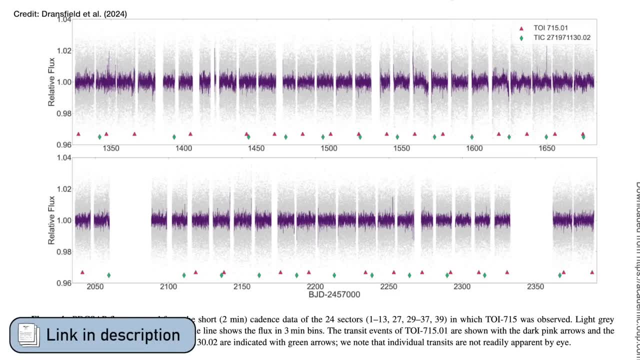 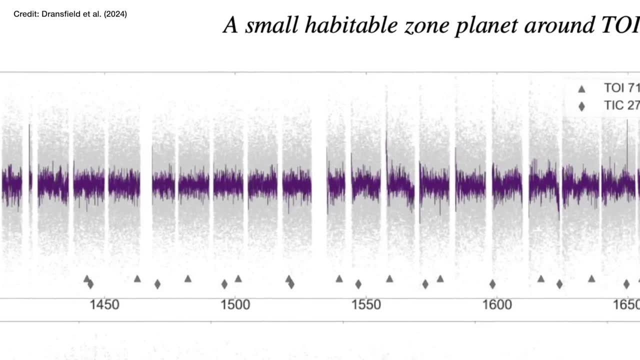 brightness data for TOI-715 over a monitoring period of about two years. The grey dots are individual measurements and the purple line shows the average of measurements taken over like three minute intervals. The red and green triangles at the bottom show this pattern of where they think. 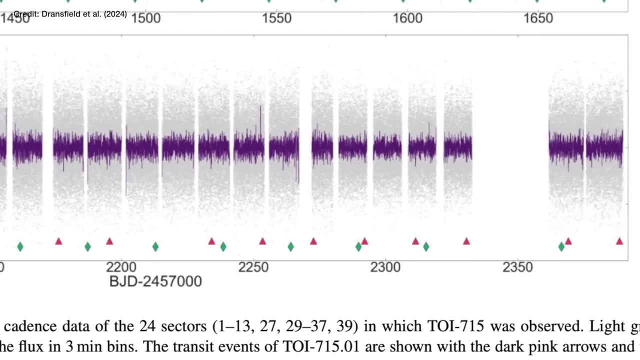 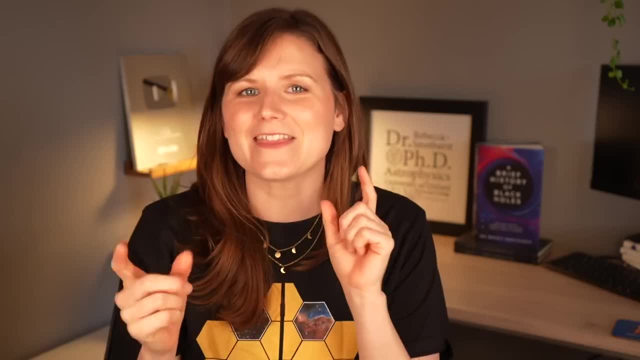 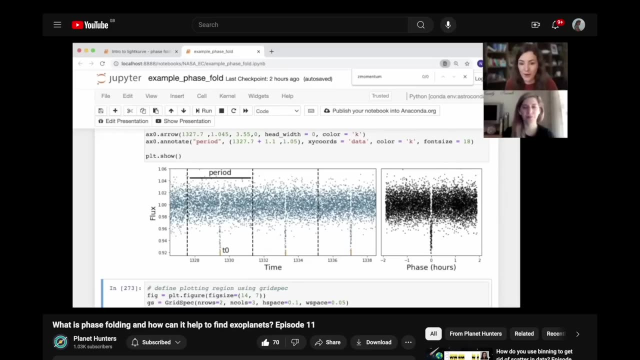 the transits of these two exoplanets have happened. Now it's impossible to actually see those transits on this scale by eye. It's only when you take the data and like fold it at the time the planet takes to orbit so that all of the transits line up, that you actually get a strong enough signal, which is 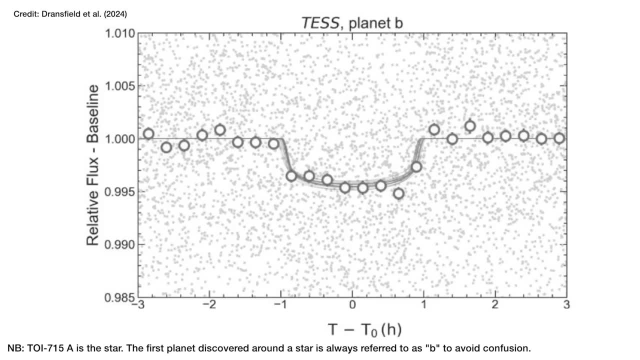 then what should happen. So that's what we're going to be looking at in the next video. Thank you for watching. Here again, the grey points are the individual observations, and so you can really see how crazy noisy this data is. but if you average the brightness in these 15 minute intervals, you get. 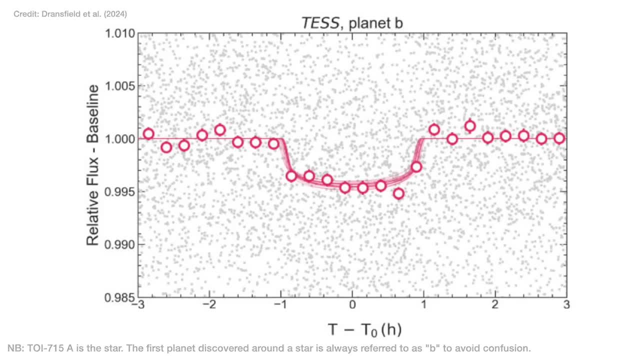 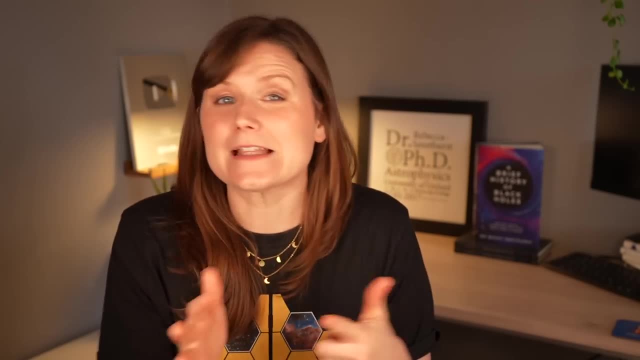 these pink outlined circles, Dransfield and collabs, then model the transit, working out what effect the planet would have on the star's light if you change its size and its mass and its orbit distance, and they get a few possible models that fit this data that are all shown there in the pink 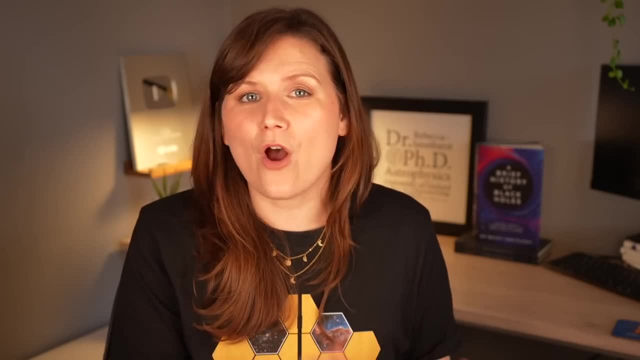 lines. Now the best fit model for this planet that they are very confident about is the TESS model. The TESS model is one of the most popular models for transits. The TESS model is a very confident of TOI-715b. is that the planet is 1.5 times the radius of the earth, orbits its star every 19 days and, from the amount of starlight that hits it, has an equilibrium temperature of 234 kelvin or minus 39 degrees celsius. That temperature is worked out assuming that the planet, like, doesn't have an atmosphere. 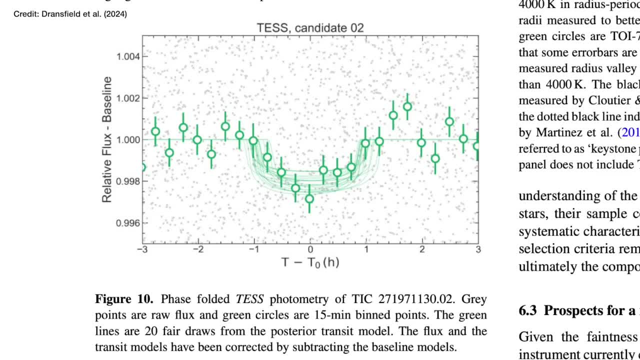 If it does, it's obviously going to be a lot warmer than that. You can then do the same for the other transit pattern that Dransfield and collaborators found Again, with the grey showing the raw data points and the green here showing that averaged data. but you can see it is a lot noisier, so they're less. 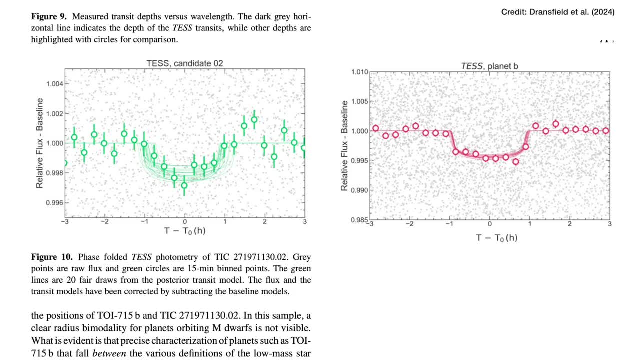 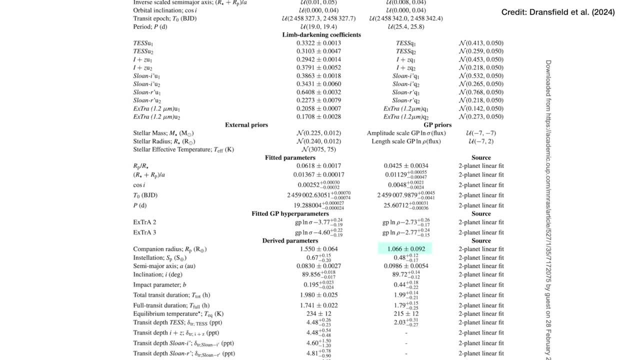 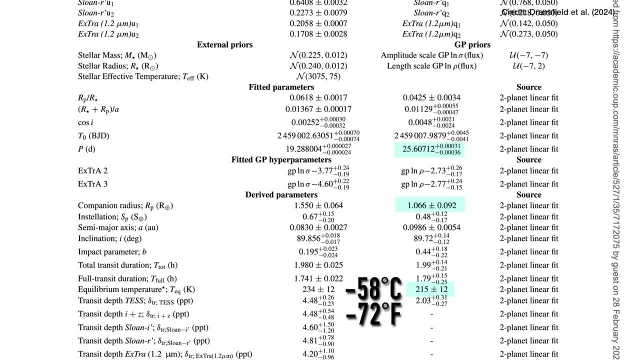 confident in the detection of this planet. But again, you can fit some models. that's what's shown in the green lines there and the best fit is that this planet is 1.066 times the radius of earth, orbits its star every 25 days with an equilibrium temperature of 215 kelvin or minus 58 degrees. 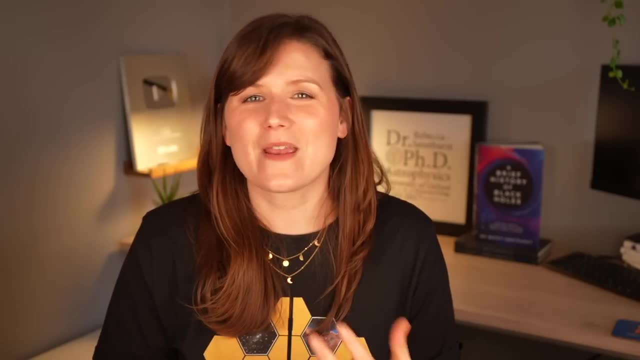 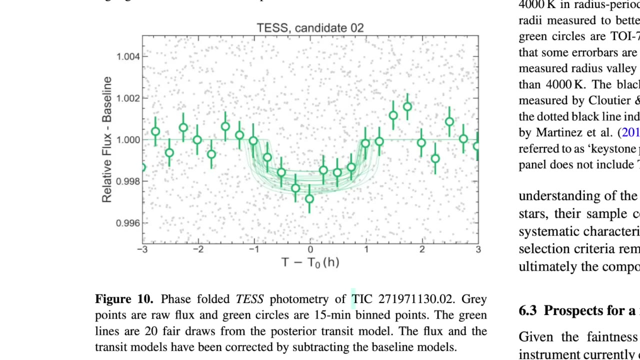 celsius, Since they're not as confident of this detection, this remains like a candidate planet, So it's a very good example of a planet for now, one that will have to be confirmed with follow-up work, which means it sadly doesn't get a name and it just gets stuck with this long number designation. 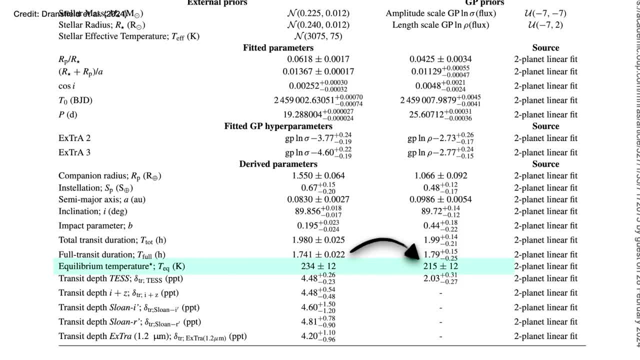 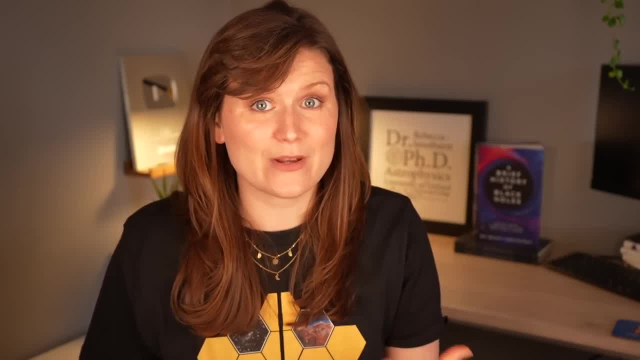 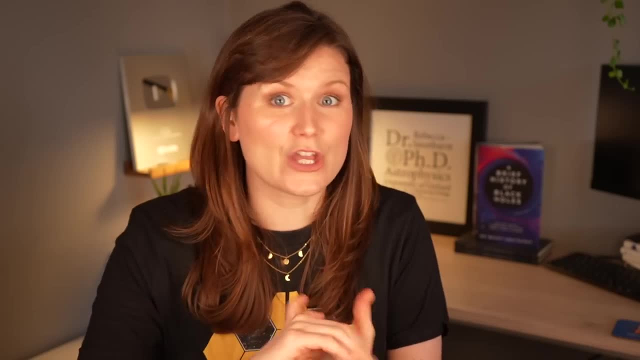 instead. Now, the temperature that Dransfield and collaborators have calculated puts this planet, and this planet candidate, well within the habitable zone around their star. So the next question is: can we use JWST to study their atmospheres? Can we work out what the atmosphere is made of, and 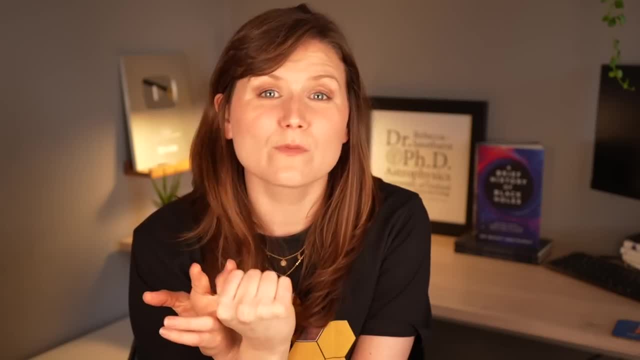 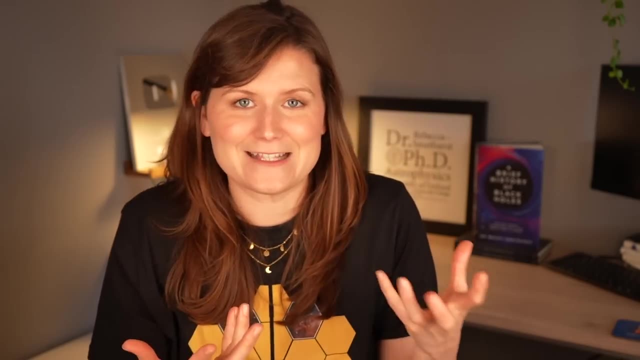 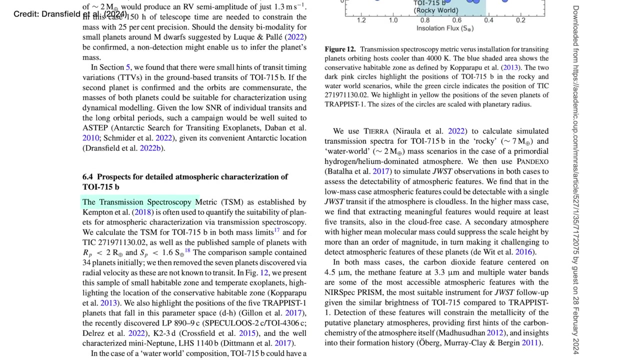 therefore like: what is the surface temperature of this planet? Is the atmosphere thick enough to support life, and are there any molecules present in the atmosphere that suggest that life might exist there, What we know as biosignatures? So Dransfield and collaborators calculated something called the transmission spectroscopy metric. It's essentially 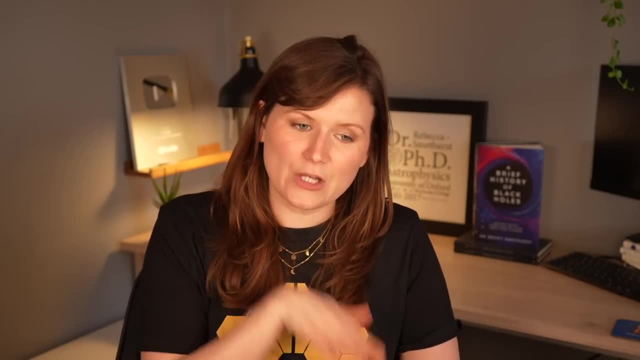 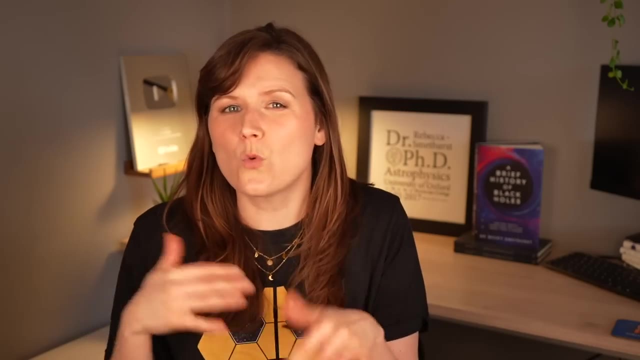 a measure of how difficult it would be to do this. The lower the number, the more difficult. the higher the number, the easier it would be. And for JWST we need that number to be above around about 12 for us to be able to study their atmospheres. So you can see in this plot the TRAPPIST-1 planets. 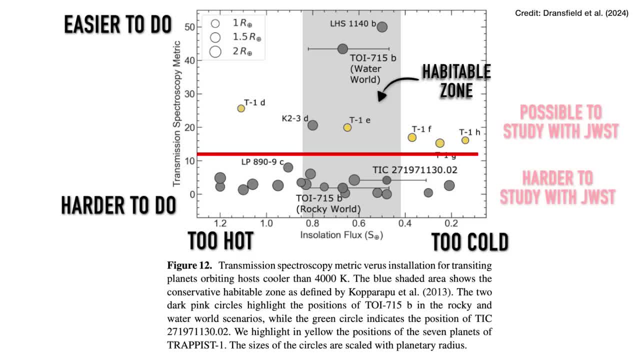 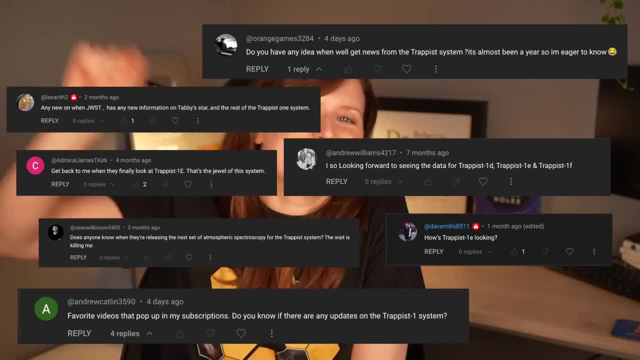 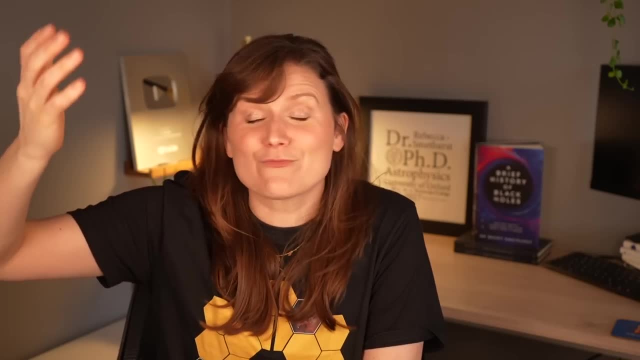 that are plotted here in yellow just about make it above that cut. So for everyone that keeps asking, like, where is the TRAPPIST-1 data from JWST? We want to see it because there's these earth-like habitable rocky planets that are in the habitable zone that we want to study, It's coming, it's just. 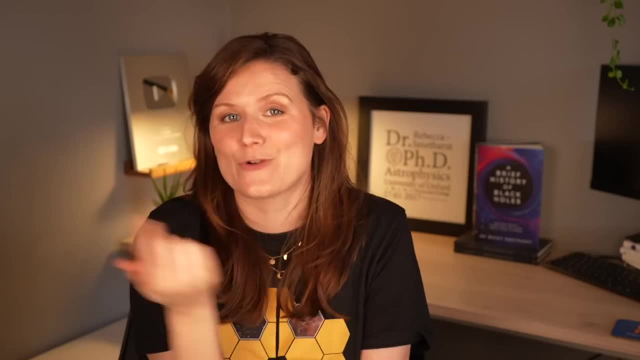 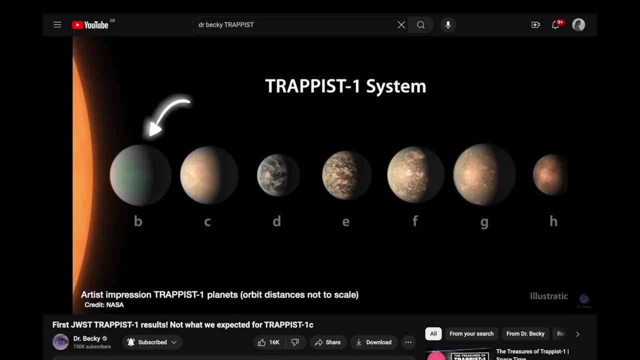 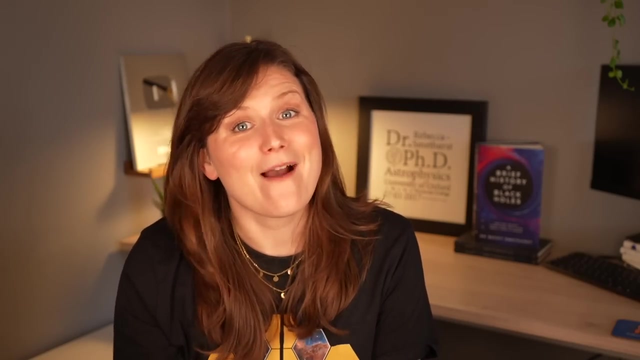 really, really difficult. You need to observe many, many transits because their metric is so low. In many transits, when JWST is busy doing other things, you have to time it properly and they obviously don't happen every day. so good science just takes time And I want it to come out to. 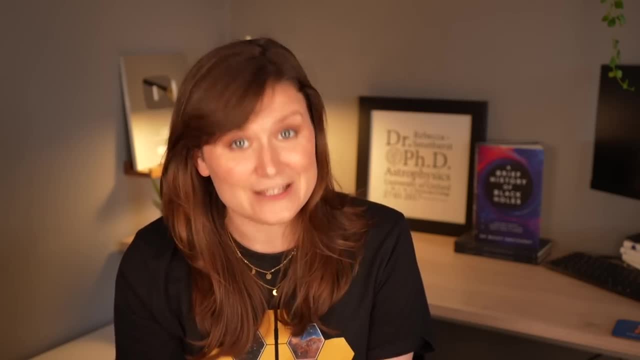 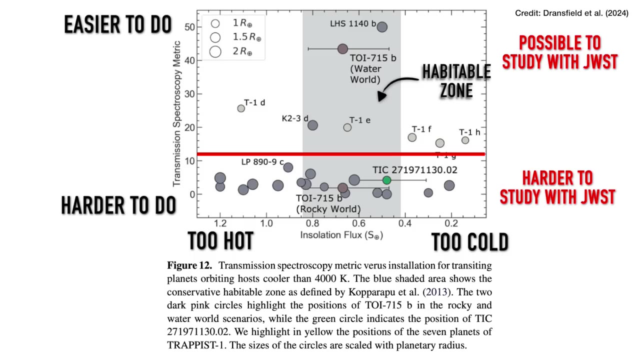 these results. okay, but it will take time. The blue points are other known rocky planets, but the points to look at here are the pink and green ones. The pink points are for that confirmed larger planet, TOI-715b, which could be a rocky planet with a very thin atmosphere giving it a